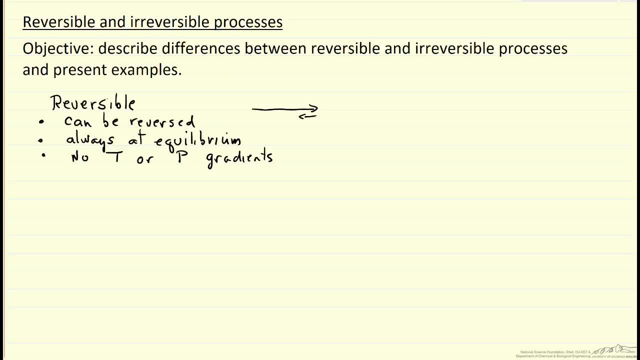 it means that the gas is pushing up 10 bar and the weight of the piston and the weights on the piston equal a pressure of 10 bar. And, of course, what we need to keep in mind is a reversible is just an ideal deal of an actual process, And so the way of comparison. 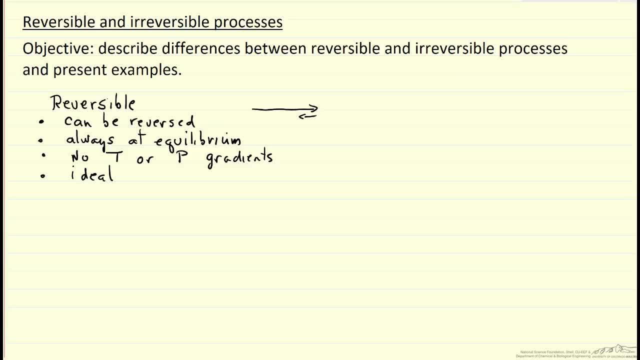 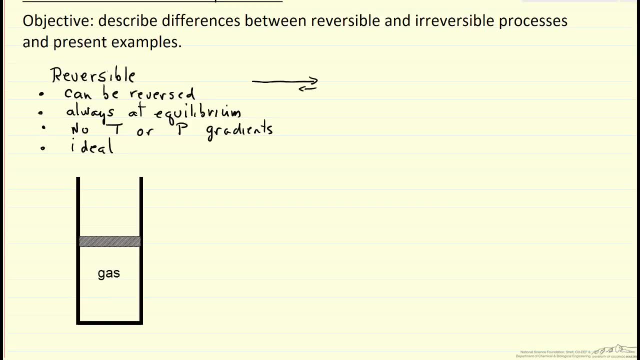 is something we make thermodynamic calculations for. So let's look at some examples to give us a little better physical feeling for what we're talking about. So let's imagine this is a cross-section of a piston and cylinder. The piston has some weight, The gas is under. 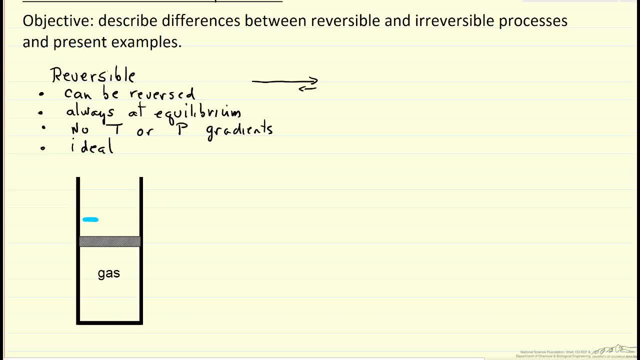 pressure in this case because sitting on top of the piston is a liquid layer And of course the liquid has some weight, so that's causing the gas to remain at that pressure, And then the weight of the liquid plus the piston creates a pressure pushing down Gas pushes. 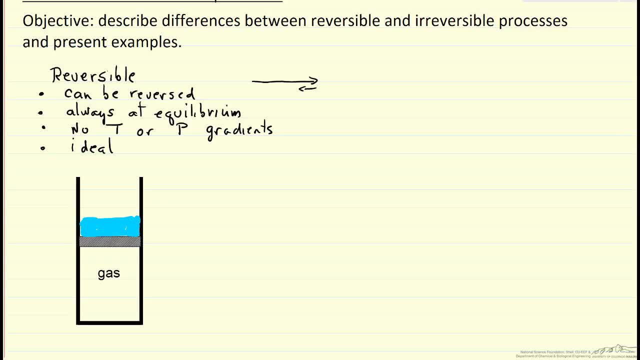 up against it at the same pressure. So pressures are balanced, Everything's at the same temperature. This is at equilibrium. So if we very slowly add more liquid slowly- so let's look at this- We're essentially think, if we're pouring in at a very slow rate, we're going to have 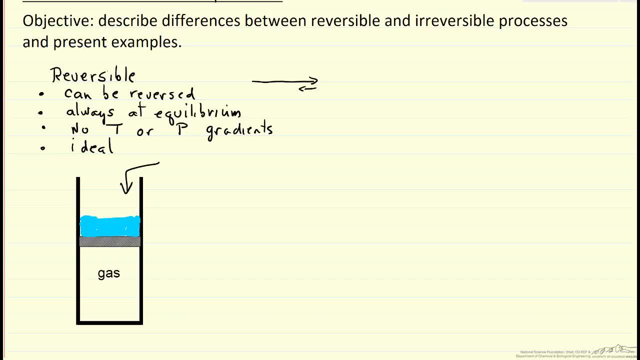 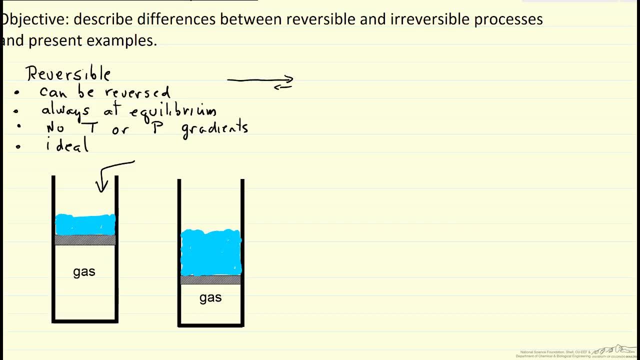 liquid. As we add more liquid, the gas is going to move down. So at a later time. so at a later time we're going to have significantly more liquid sitting on top of the gas. The gas is going to be at a higher pressure. It's in equilibrium. You can imagine at any instant. 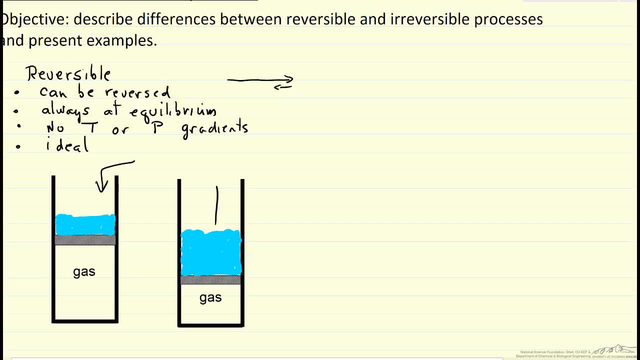 we could just reverse this and start removing liquid. It could be as simple as some small valve on the side. Very slowly start taking liquid out instead of adding it Now. the gas pressure would decrease, The gas would expand. We're doing here everything isothermal. We could be doing everything adiabatically. The result: 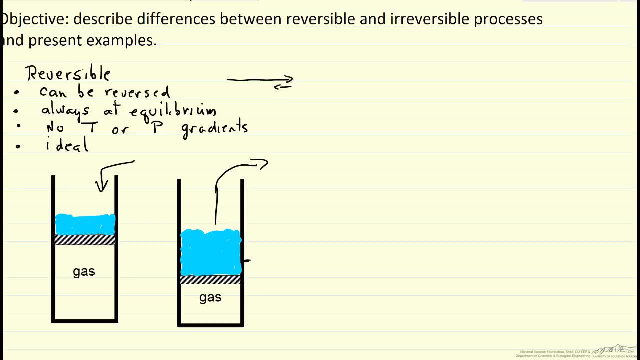 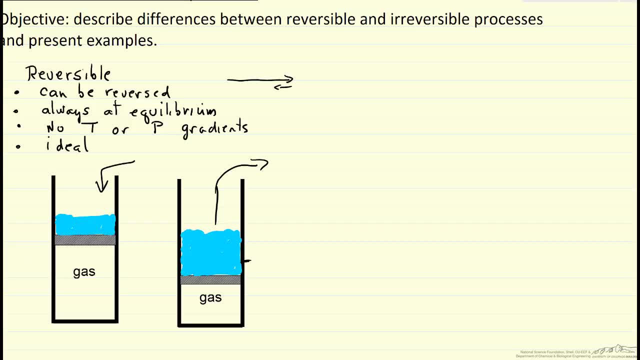 it at a very slow rate, So we're always doing it at a very slow rate, So we're always doing it essentially at equilibrium. So it's a very good example of what we mean by reversible process. Let's look at another example of a reversible process. Here we're looking at a single component. 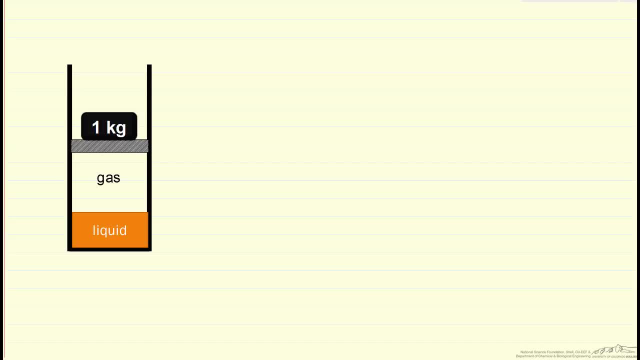 at vapor-liquid equilibrium with gas or vapor It inequilibrium with the liquid. The pressure is constant. It's indicated by a weight, say on a piston, that we don't change Slow. So if we were to add heat to this we would start evaporating some of the liquid into. 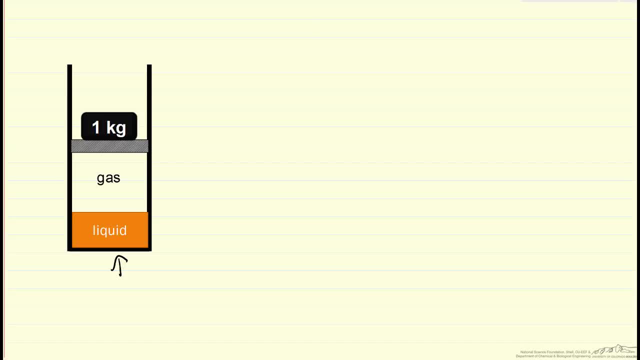 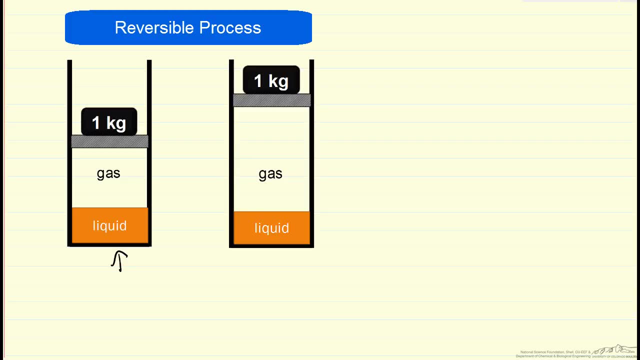 the gas phase, the piston would move up. So then, at a later time, we'd have more vapor, more gas. we'd have slightly less liquid, since gas occupies a lot more volume than liquid. Pressure's the same, The temperature's the same. 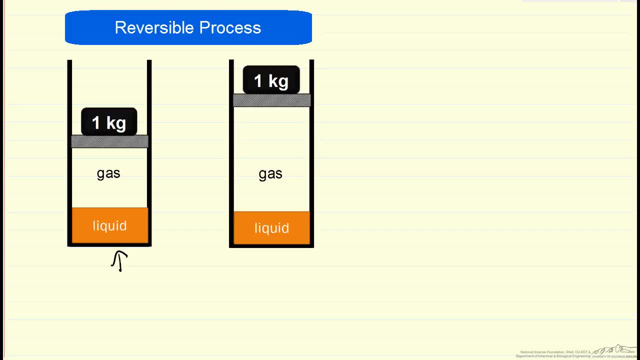 And the fact we added heat doesn't change the temperature, because at constant pressure, single components are going to evaporate at one temperature, And so, as we continue to add heat, we maintain vapor-liquid equilibrium. We have no pressure gradients. We have no temperature gradients. 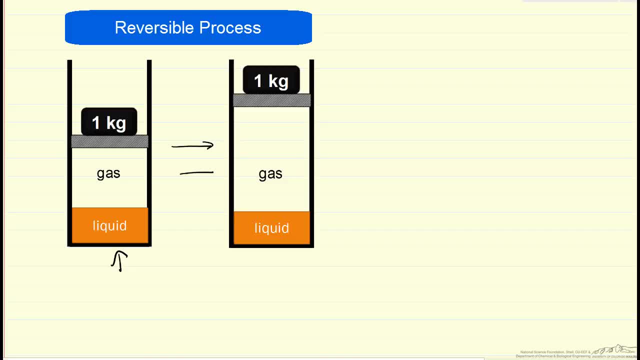 And so this process is reversible, in that, at any time, we can start going in the other direction. If, instead, we start removing heat, Removing heat from this system, we're going to end up eventually back at this system. Every step of the way is in equilibrium. 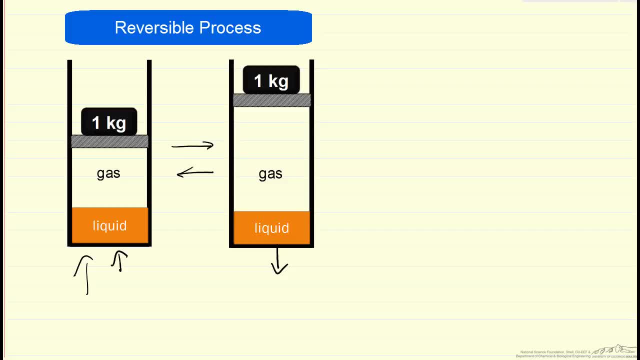 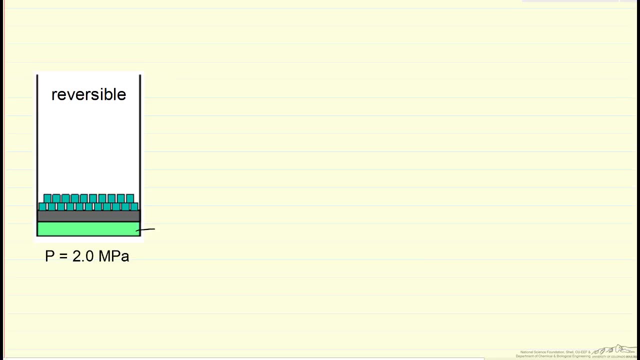 So vapor-liquid equilibrium, single component, constant pressure- very good example of a reversible process and something that we can do practically. Now, if we look at, let's go back to single components. So now we have gas. We have gas. 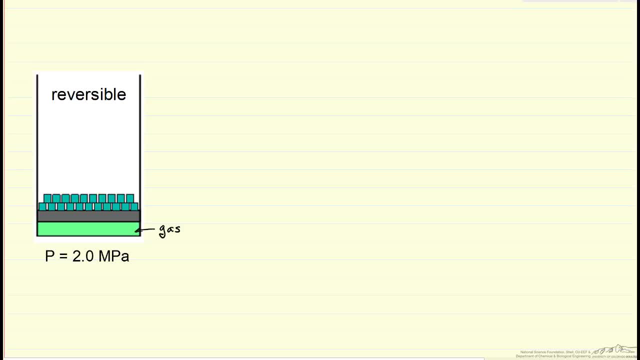 We have vapor, We have liquid, We have liquid canola, high pressure And a reversible expansion. for example, a reversible adiabatic expansion would be the system be insulated- and I've drawn a bunch of weights on the top of the piston. and if 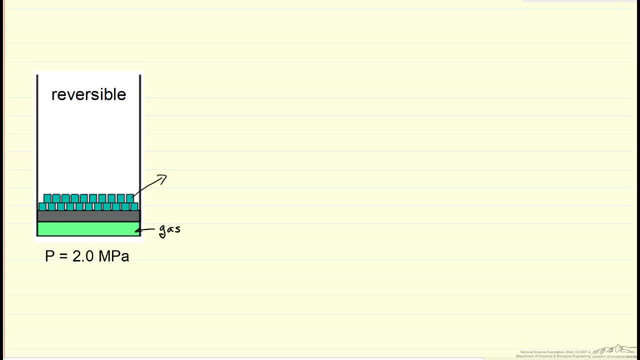 I start taking off one weight at a time. first weight's taken off, The gas expands slightly. Take off another weight, Expand slightly more, But these weights are very small, So I have a very large number of them. then I am close to a reversible process, the equivalent. 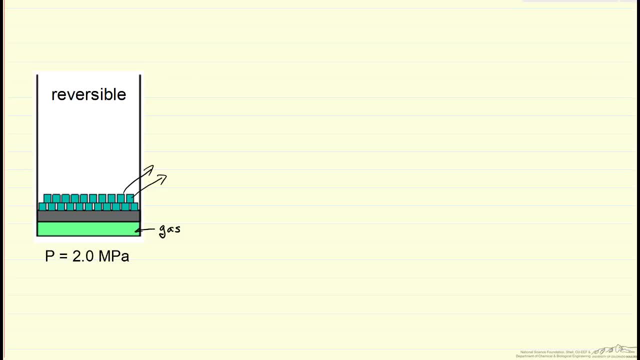 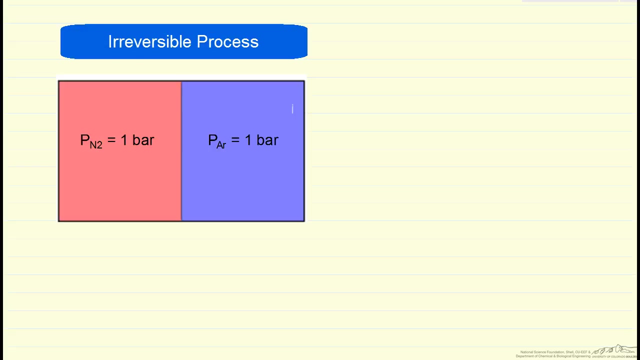 of the liquid which I can imagine removing incrementally very easily. This is then an approximation to that liquid of a reversible process. What would an irreversible process look like for gas expansion? Let's look at one more example of an irreversible process. Here we imagine two containers at the same pressure but with different gases, and they 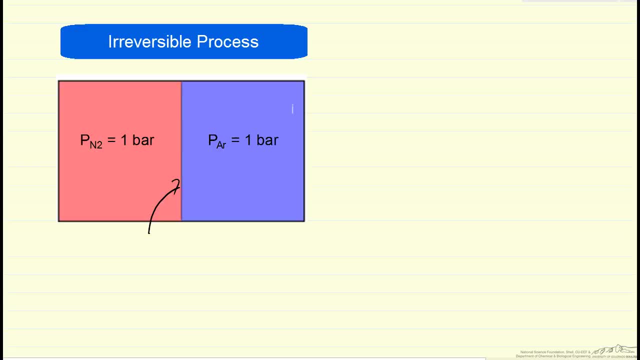 are separated by some thin diaphragm. If I could quickly remove this diaphragm or punch a hole in the diaphragm, what's going to happen is nitrogen is going to diffuse in this direction, because there is no nitrogen on the right side. 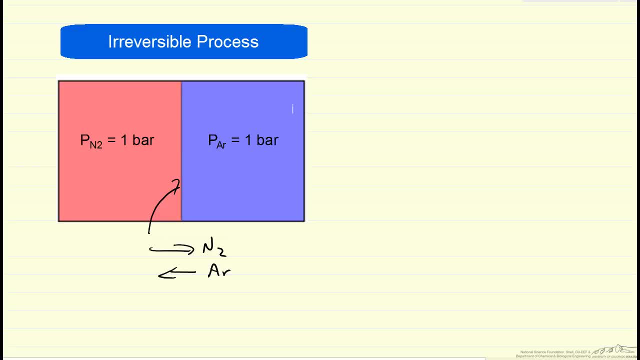 And argon is going to diffuse in the opposite direction And they will keep doing so until the partial pressures are the same. if we instantaneously remove the diaphragm- and we can imagine doing that- they would much more quickly diffuse until the pressure of argon. the partial pressure is a half a bar and the partial pressure 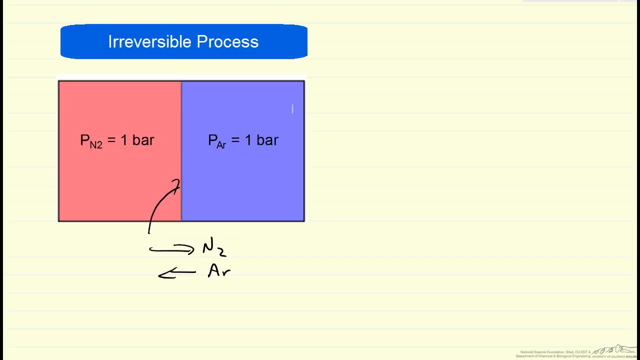 of nitrogen is a half a bar, since they are the same volume. So they are going to diffuse in the opposite direction And argon is going to diffuse in the opposite direction And they are at the same pressure, Clearly irreversible, because we can't at any point stop and go in the other direction. 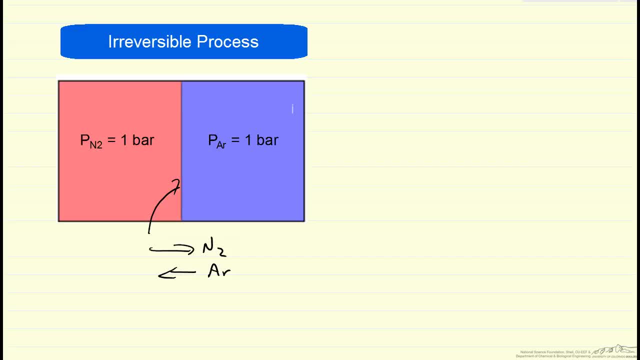 So it's a good example of what we mean by an irreversible process.